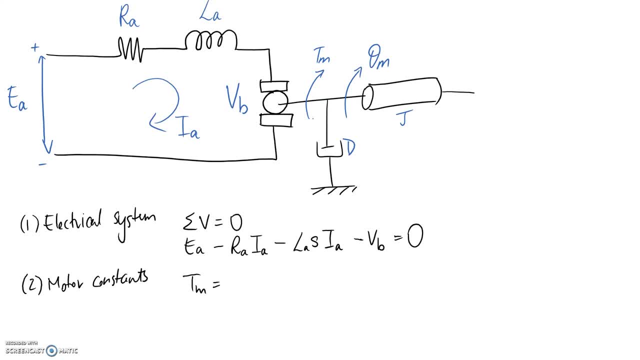 use for this. so the first one is that the torque out of your motor, which i've already labeled here, is equal to kt, which is the torque constant multiplied by ia, which is the current again running through this circuit. so to be able to substitute this back up into the other equation, 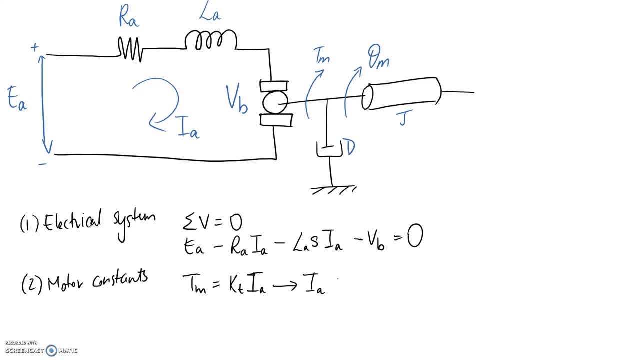 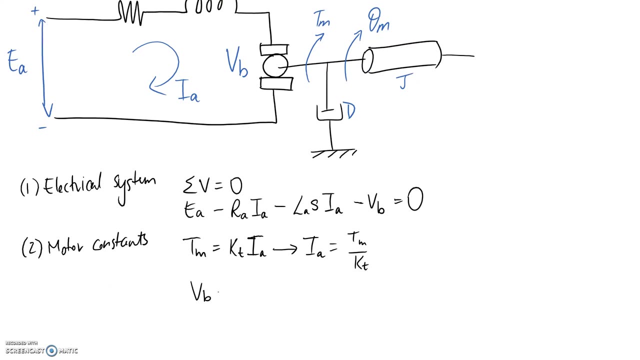 we're going to need to rearrange it in terms of ia so that becomes tm on kt. the second equation that we're going to do is to substitute in our motor constants, so that's our second equation to have is that the voltage, vb is equal to kb times theta dot m, and if we want to, we can go ahead. 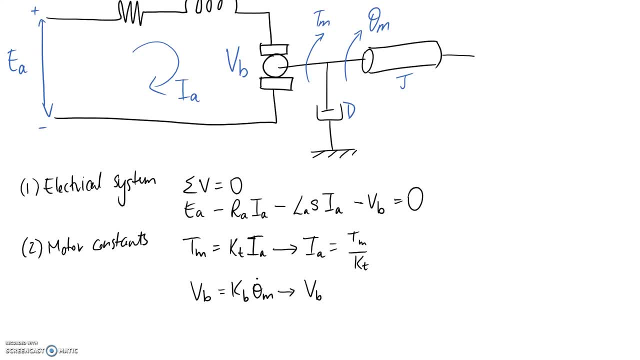 and look past. transform this, oops sorry. vb then is equal to kb. transforming this, it becomes s, theta m. one dot means we get one s, so you can either substitute them all at the end of the equation or you can do it progressively. i might go ahead and do it now, so let's put these two. 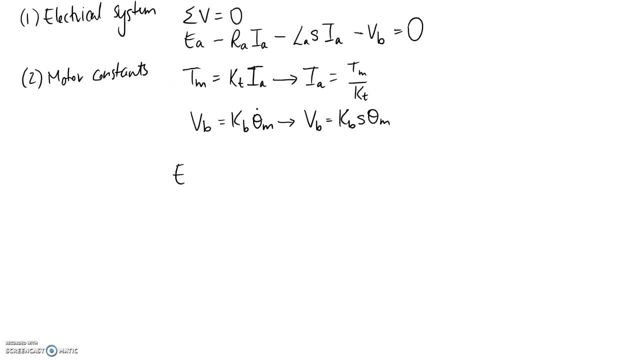 back up into our first equation. all right, and i might factorize this a little bit to make it easier in a moment. so i'm going to put um, these two terms kind of together and take out the tm. so what i'm going to get is ra plus las. 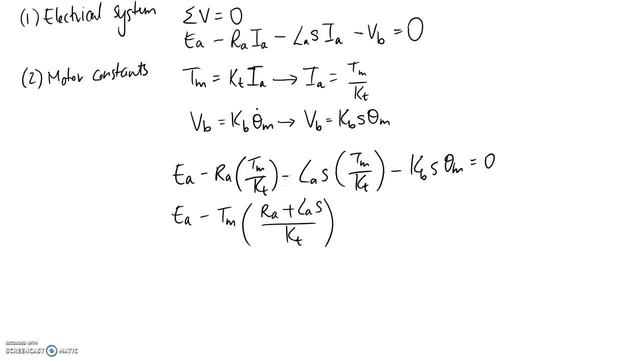 on kt in the bracket. if you expand that out, it should be those two terms, all right. so to be able to keep going, we need our third equation, which comes from the rotational system. so for that we're going to need to draw a free body diagram of our system. 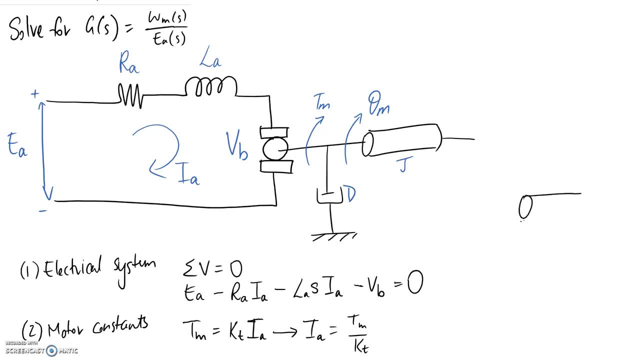 so let me do it over here and then I will transfer it down, So taking out the body and marking on some things. So we've got torque applied in this direction and that's the torque from the motor. We then need to assume a direction that this thing is going to rotate in. 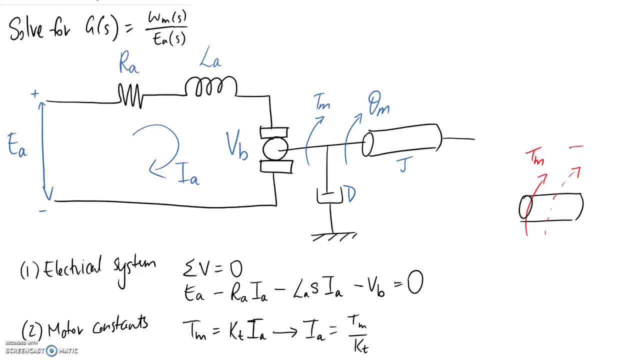 and I'm going to assume it's going to be the same way, So it's going to be J, the inertia multiplied by the acceleration, or the angular acceleration, which is theta double dot m, Remembering this is theta m already marked in. and then we've got a damper that's applying torque onto the shaft. 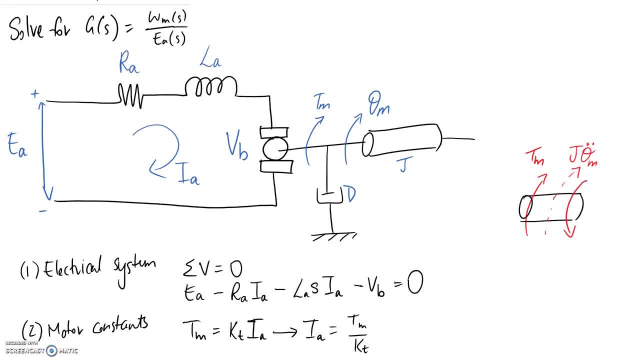 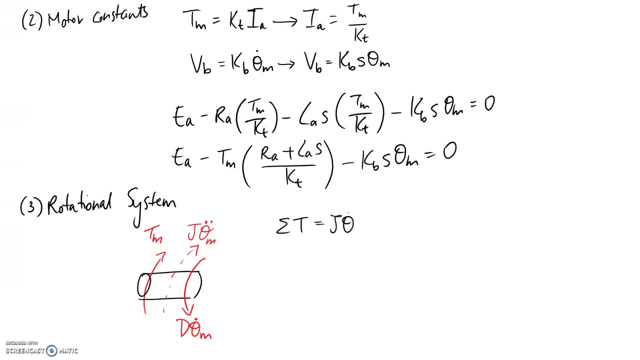 and this is going to try and oppose the direction of motion and slow it down. So it's going to be the opposite direction. It's going to be d multiplied by the speed of the shaft, which is theta dot m. All right, so I've just copied that down here so we can keep going and the equation: 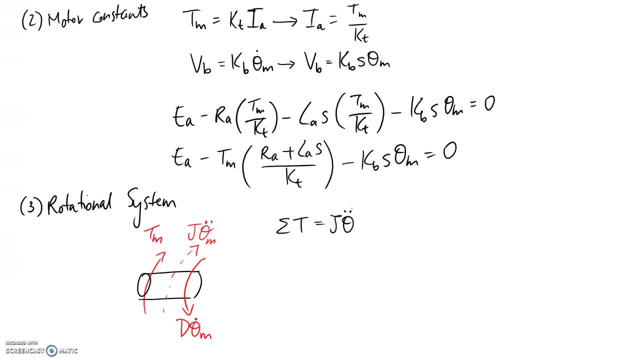 that we need to do is we're going to multiply the speed of the shaft by the angular acceleration. So I'm going to multiply this by the speed of the shaft, which is theta double dot m. so we're just going to take the giving this a little bit of time, and this is the same thing we did for the column. So I'm going to 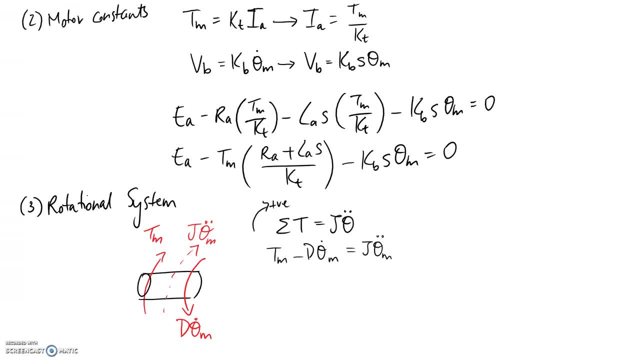 put this on the left of the equation and this side is going to be the weakness and I'm going to put it in the positive direction. so I'm going to put it positive in the equation. So now what I want to do is rearrange this. I'm going to leave torque on one. 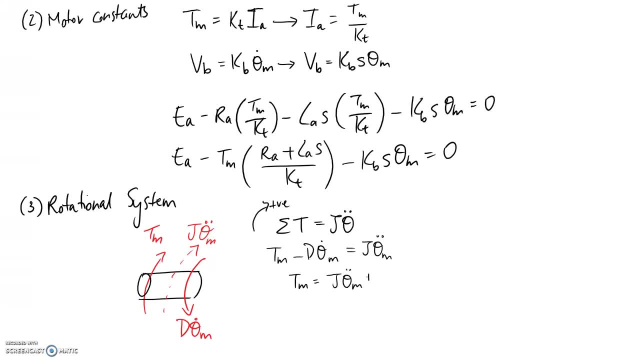 side and move everything else to the other, and that's because they both have the theta term in them. and then what I want to do is transform this. so tm is a function of time. when we transform it, it's going to become the whole pass of itself. we would capitalize it, except I already wrote it. 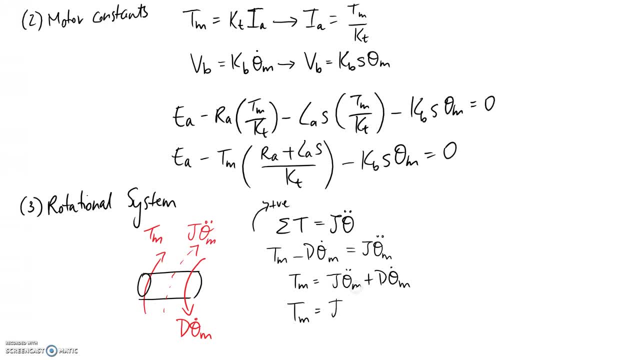 with capital j is a constant, so it stays out the front. when we transform this, it's going to get an s squared times theta m again. this is the one that gets transformed. I would capitalize it, but it's theta. it's kind of hard. and same thing for 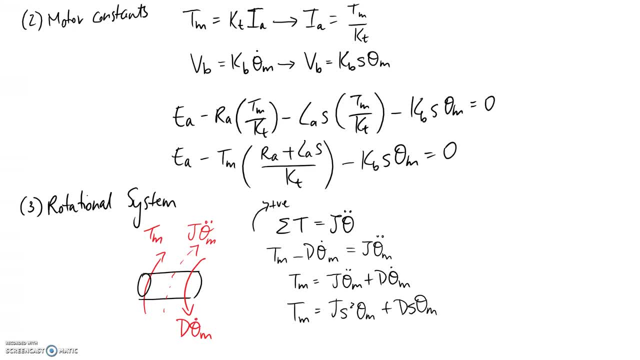 this one. I should quickly mention that we're going to assume all the initial conditions are zero, so there's no initial displacement and no initial velocity and things like that to consider all right. so the last thing I want to do here is I'm going to factorize out the theta m. 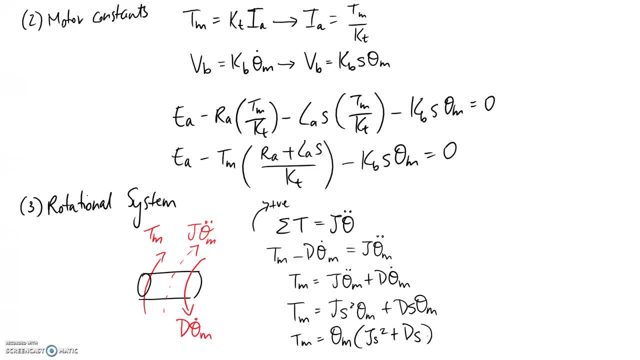 and that's what we end up with. so now, what I should be able to do is substitute this equation back up in here, and it's going to eliminate tm from the equation, and the only variables should then be ea and theta m, which are directly related to that transfer function. I'm going for. 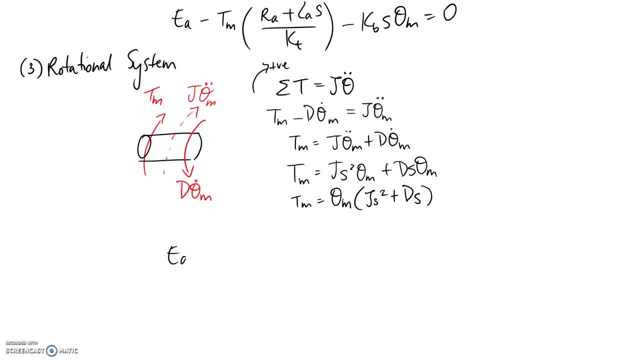 so let's sub it in and we get that. now what I'm going to try and do is move the two things with theta to one side and leave a a where it is, and at the same time, I'm going to factorize out the theta m. 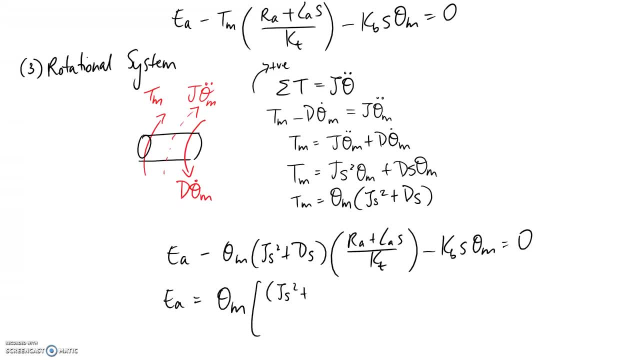 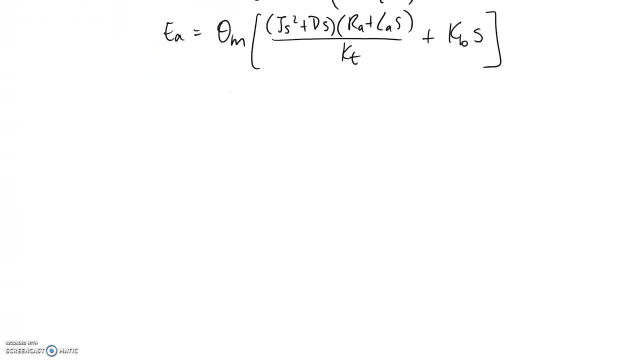 oops, sorry, I missed the j's okay, so that's what we're left with now. if I want to, I can make this a little bit nicer. I can see I've got kt here, so I can kind of integrate this with this other term and one way of doing that. 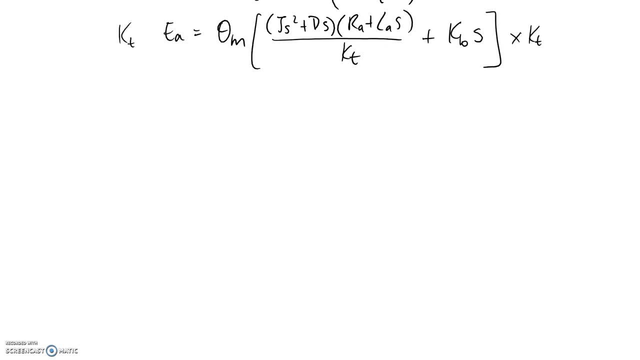 would just be to multiply both sides by kt. okay, so this becomes ea, kt, this one. so kt divided by kt. it's just going to disappear, and then kbks times kt. we end up with that so that looks a little bit nicer and remember the transfer function that I'm going for if we scroll all the way. 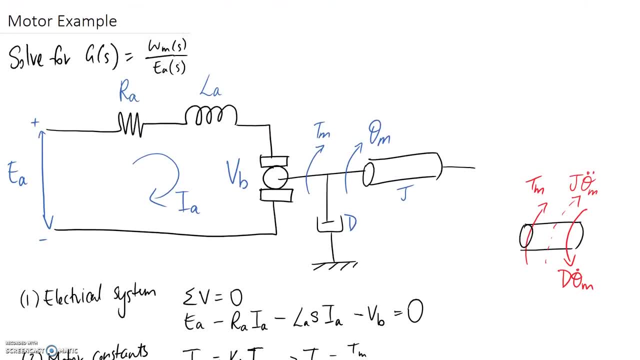 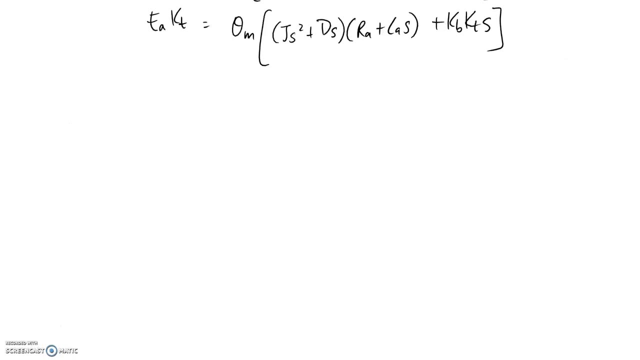 back up was omega m divided by ea, and we're going to be able to evaluate omega m back to theta m quite easily. so at this point in my process, what I'm going to try and solve for is theta m divided by ea. so, coming back down, 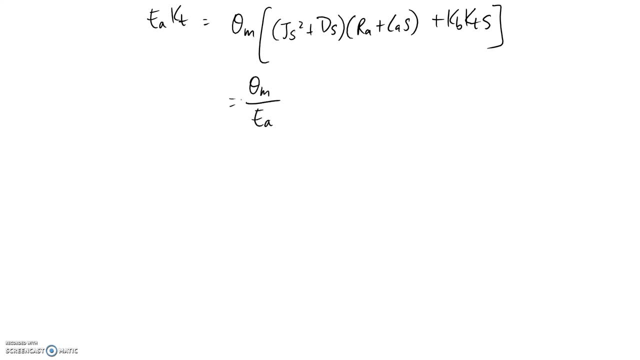 so c to m divided by ea. I can get quite easily. I just bring this down to the other side of the equation and I'm going to be left with kt on this side, divided by all this. okay, so now the last bit is to try and change this. instead of theta m,